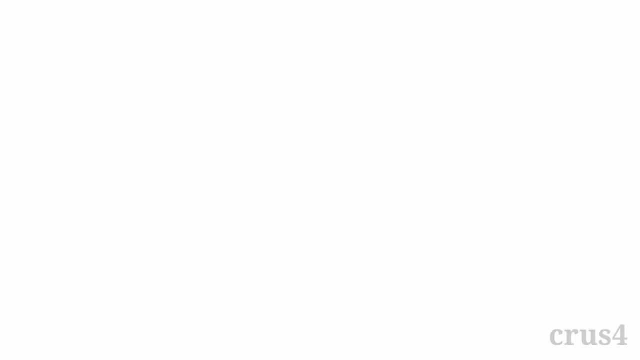 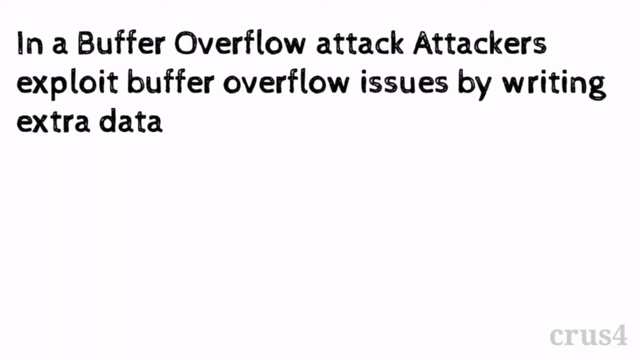 This is what buffer overflow is in brief. Now, in a buffer overflow attack, attackers exploit buffer overflow issues by writing extra data which holds specific instructions for actions intended by a hacker. For example, the data could trigger a response that damages file, changes data. 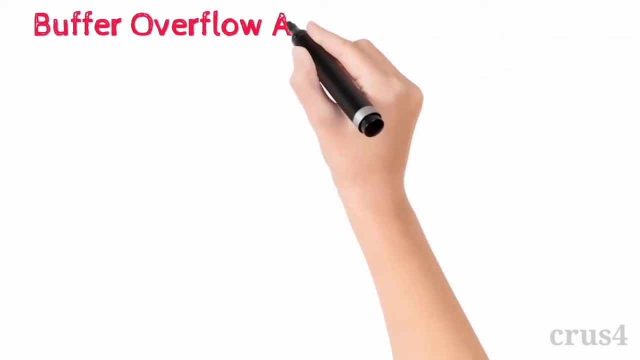 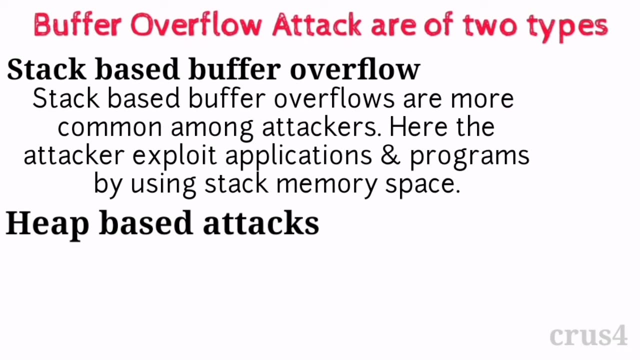 private information. Buffer overflow attack are of two types: stock-based buffer overflow and heap-based attacks. Stock-based buffer overflows are more common among attackers. Here the attacker exploits applications and programs by using stock memory space, which is used to store users' input. 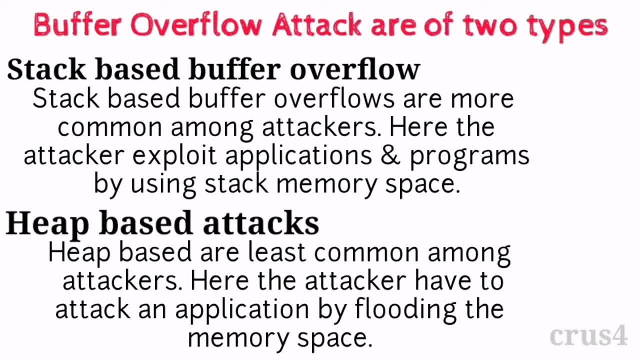 while heap-based are least common among attackers. Here the attacker have to attack an application by flooding the memory space reserved for a program, and it is also difficult to execute. So these are the types of buffer overflow. Now let's discuss about how you can prevent buffer. 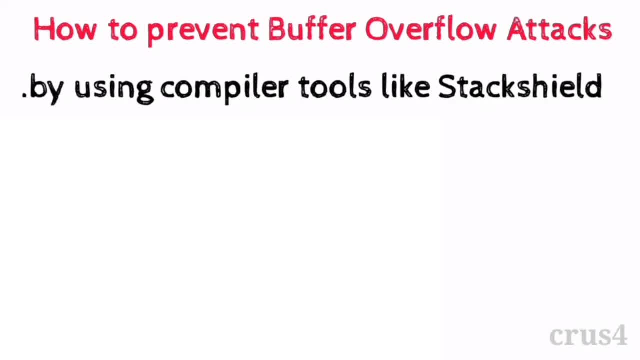 overflow attacks. We can protect against buffer overflow vulnerabilities by using compiler tools like stock shield, stock guard and heap-safe, Or by using safe functions like stransp, and also by code auditing. Now, at the end, let's take a short look at the summary of this lecture. 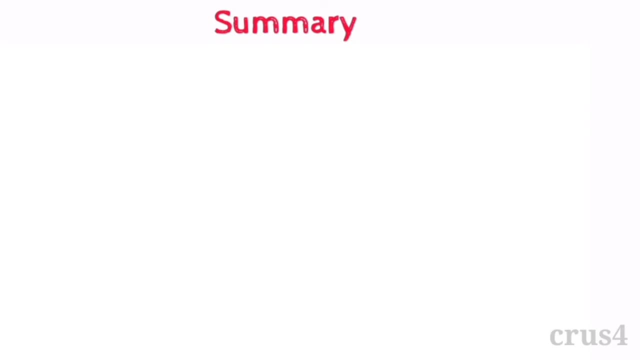 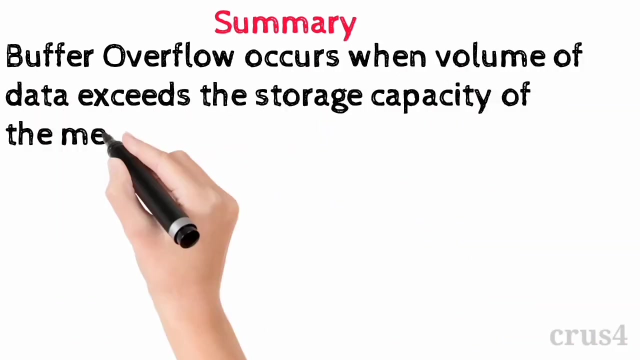 So in this lecture we have learnt about buffer overflow attack, where we firstly discussed about buffer overflow, which occurs when the volume of data exceeds the storage capacity of the memory buffer. For example, if you are filling a form on a website and a maximum character error for 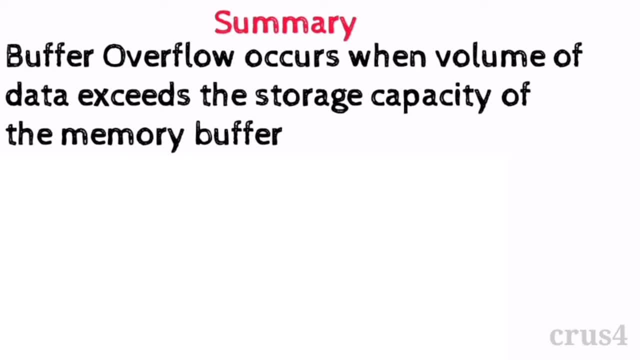 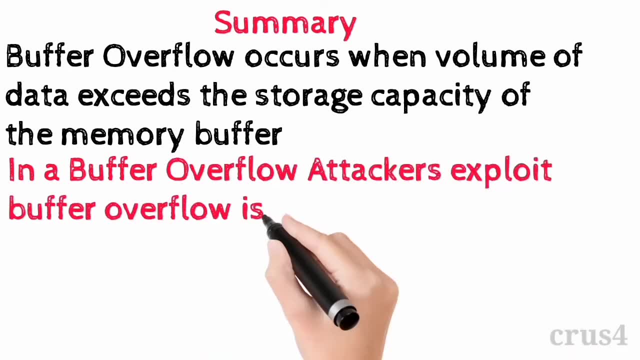 the password is 10, and you enter something extra longer than 10 characters. so here the buffer overflow occurs Now in a buffer overflow attack. attackers exploit buffer overflow issues by writing extra data. Buffer overflow are of two types: stock-based buffer overflows and heap-based. 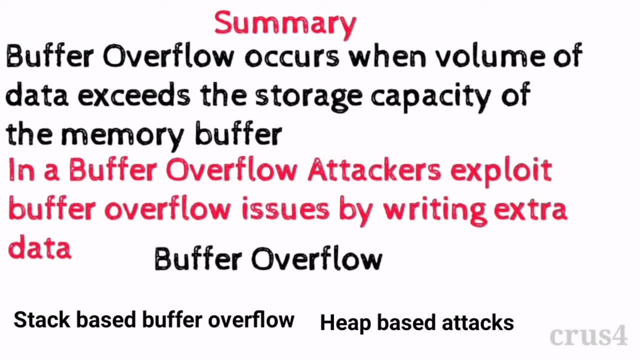 attacks. Out of these two, stock-based, are more common among attackers. We can prevent buffer overflow by various means, which includes using compiler tools like stock shield or by using safe functions like stransp, and also by code auditing. If you want a practical on this, let me know in the comment section. So that's it for this video. 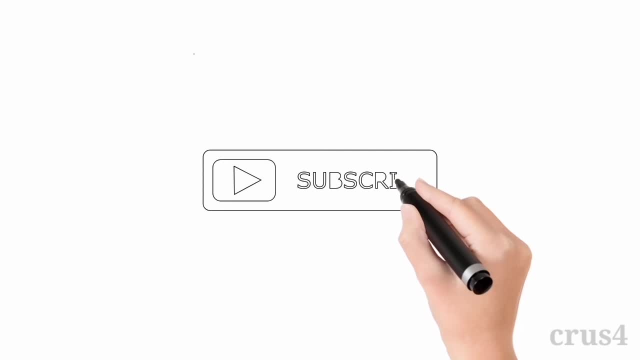 I hope you guys like it. like, share, comment and don't forget to subscribe watcha cresspo for more informative videos related to technology, ethical hacking, cybersecurity and programming. See you next time. Till then, thank you and bye-bye.